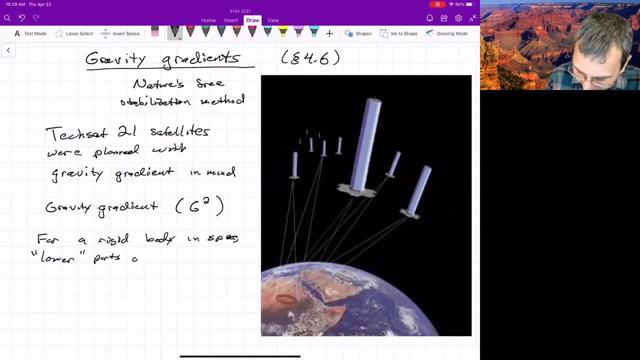 the middle of the earth. the lower parts of the body have a stronger gravitational force than the upper parts, which leads to restoring torque. But then it gets complicated. We've got 3D shapes here. We might say the lower parts are heavier, which is utterly confusing. Heavier, Yeah. 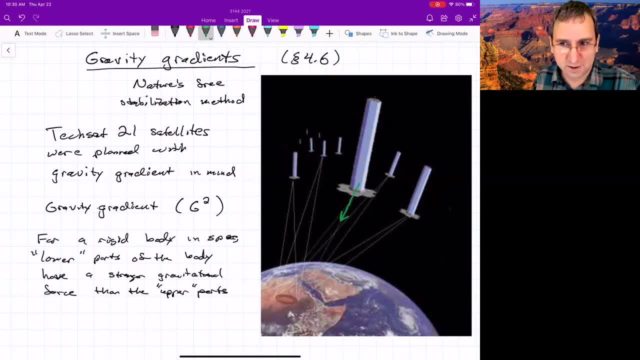 So right, The force of gravity is what we call. you know, something's heavy or not heavy. This is heavier than up here, So that force will be less. Of course, we're abstracting this as if all the mass is concentrated at the bottom and the top, And it's not, It's throughout, And we're going. 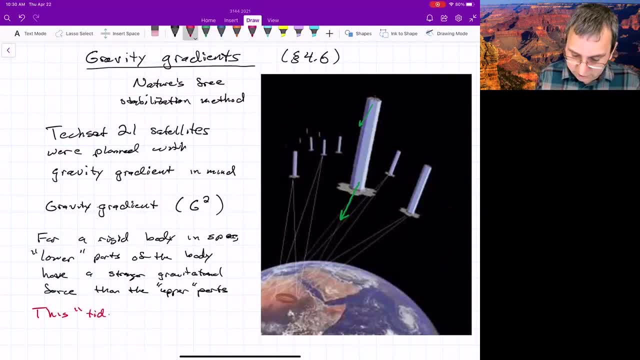 to have to take that into account. So this force will produce a torque on the body. It's sometimes called the tidal force And you might wonder: well, why don't we use gravity Gradient stabilization for everything? like something up in the air The torque is really. 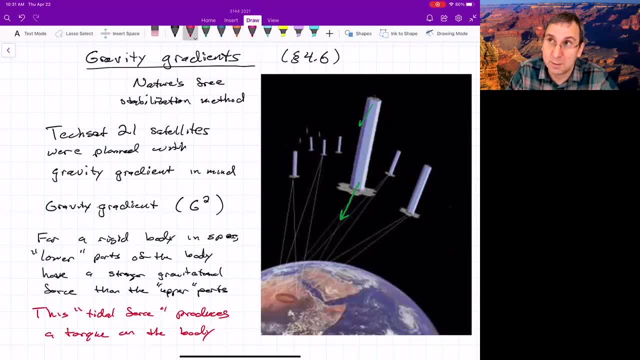 small. It's really small, So it would be dominated by like wind up in the air, But when you're out in space it's vacuum. So this torque- it could be significant enough that it works. So how does it work? We're going to have to back up and analyze this situation in a careful way, So let's talk. 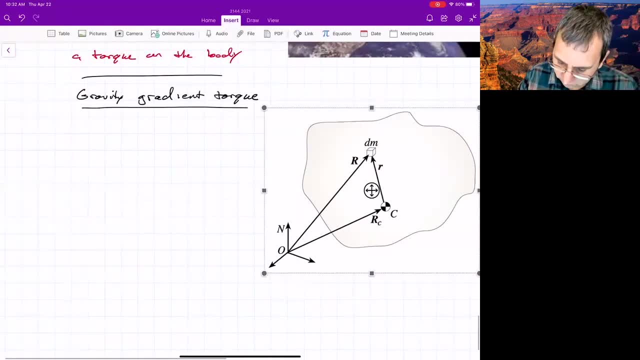 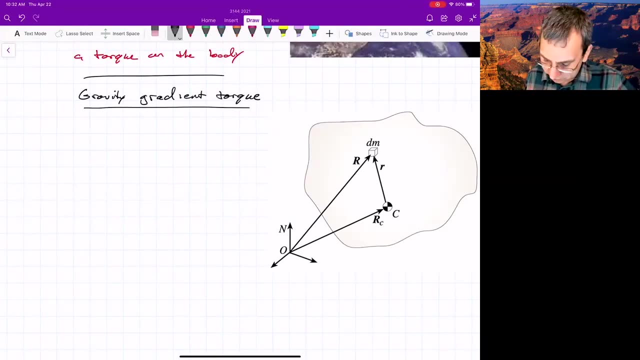 about what that gravity gradient, torque is. It's good at this point to have an image, Image of an abstract body. So we've got mass elements, We've got an inertial frames, So this would be center of earth, And then we're using some inertial frame center to the center of the. 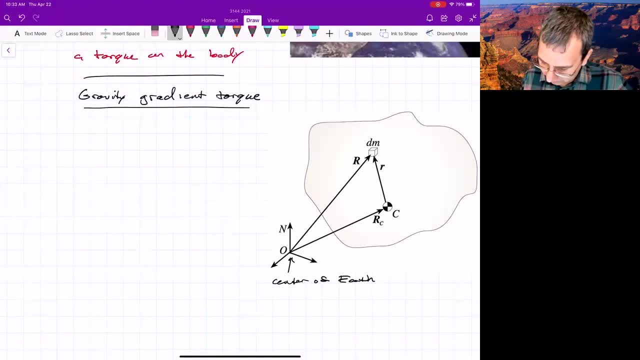 earth fixed relative to the fixed stars. The location to the center of mass is RC And the location to some point in the body is capital R. Little r represents the vector from the center of mass to the little mass point. So we've got this inertial frame. 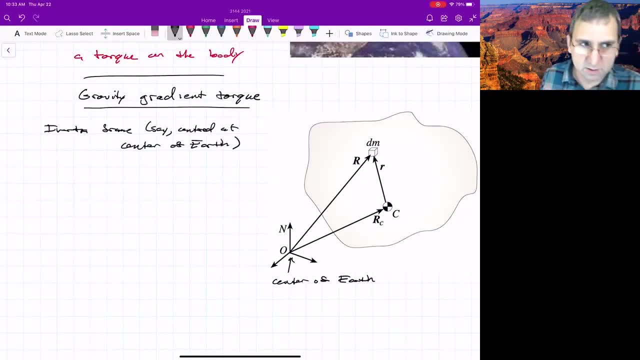 Say centered at center of earth, But really it's just sort of the massive body that you're around Like. people might be working on trying to do gravity gradient torques for satellites around asteroids, In which case it's not centered at the center of the earth, It's centered at the 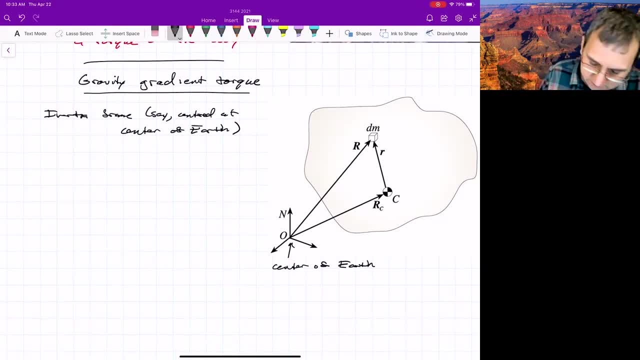 massive body you care about, But for now let's think of things about the earth. So this is: we've got our inertial frame, And I'll just say it's got an origin O And then the usual N1, N2.. 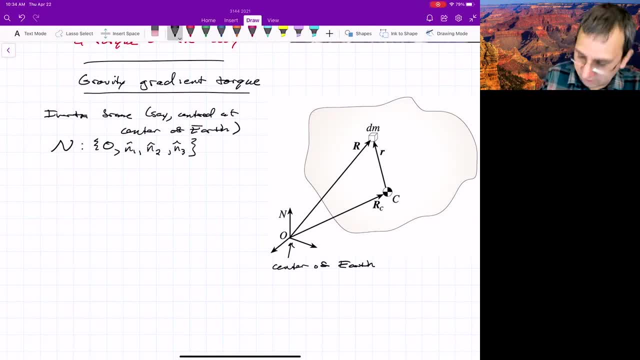 And 3. We've got inertial vectors. Those are an RC, And then the relative vectors, little r. So I'll just note that that location, this is location of mass element dm with respect to inertial origin, Or let's just say origin O, And that's going to be location of the center of mass. 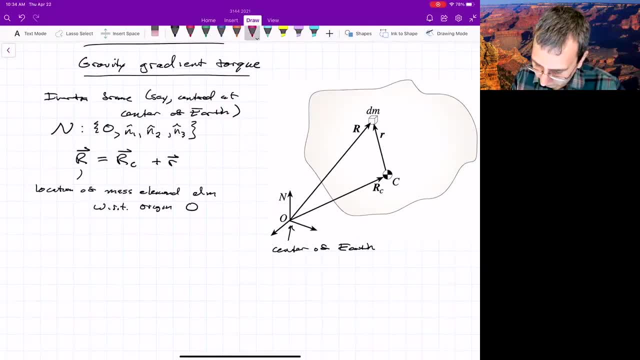 of the body plus little r On the mass element. so here's our mass element. there's going to be a force And because this is gravity, it's going to be going towards the inertial origin. here We'll call this df. It's the differential force of gravity on that element And dfg is going to be. 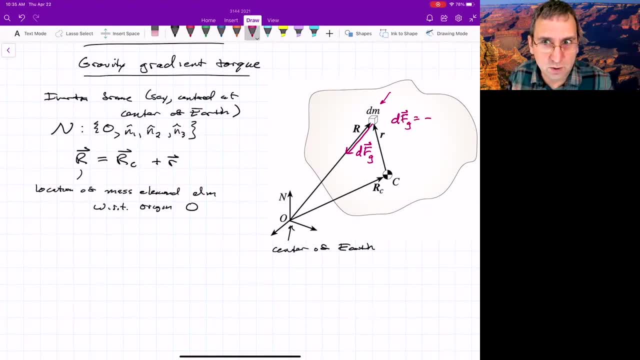 equal to- and now you need to use what you got from orbital mechanics: capital G, gravitational constant. mass of the earth, mass of our little element Divided by the distance to the center of the earth squared, There's that negative sign. 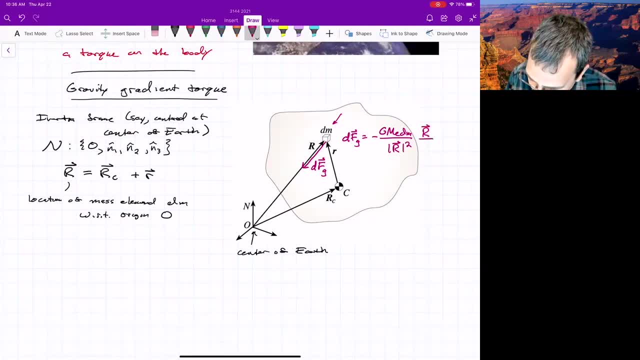 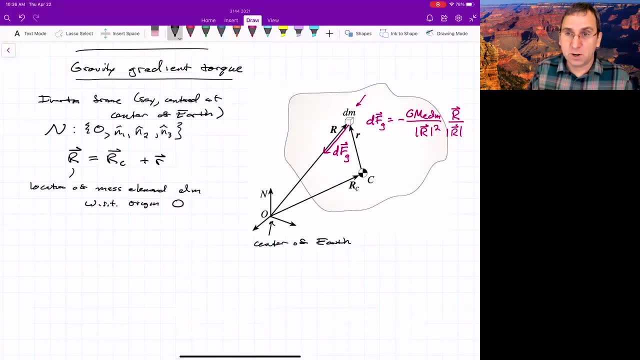 meaning it's pointing in the negative r divided by magnitude of r. So it's pointing in the negative radial direction, Super. Now we want to know what the gravity gradient torque acting on the spacecraft. It's called gravity gradient because the effect of gravity isn't the same throughout. 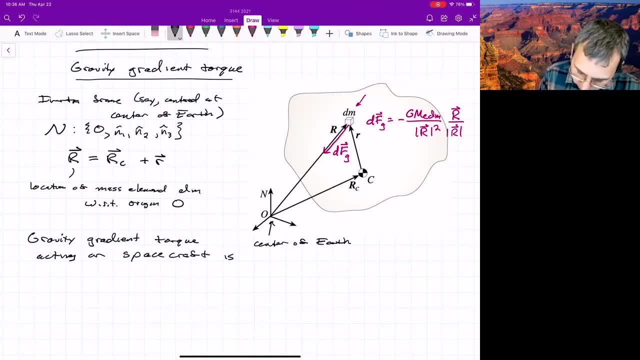 There's a gradient, And we will call that l sub g. This doesn't mean well, it means torque due to gravity. And what would it be? We would be doing an integral over the body. So this is the body of r cross dfg right. And then what's that going to be? We can 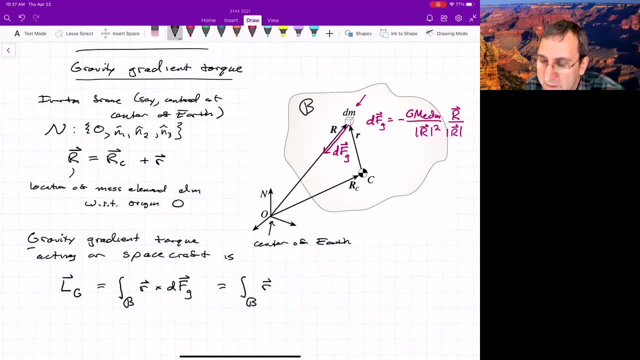 substitute in what we know for dfg. so it'll be. let's put the minus sign out in front and this will be r cross. this is the cross product vector. cross product g and mass of the earth- i didn't say it me is mass of earth, or whatever the body is that you're about, and then, uh, put magnitude of r. 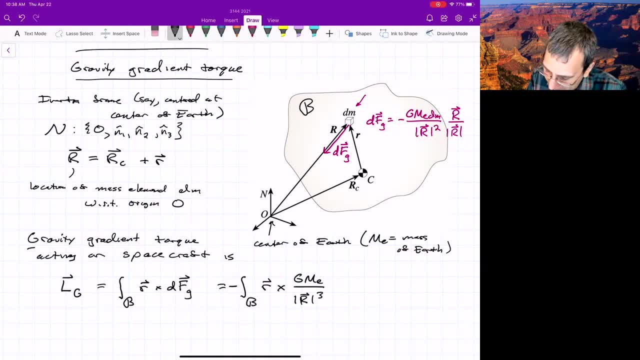 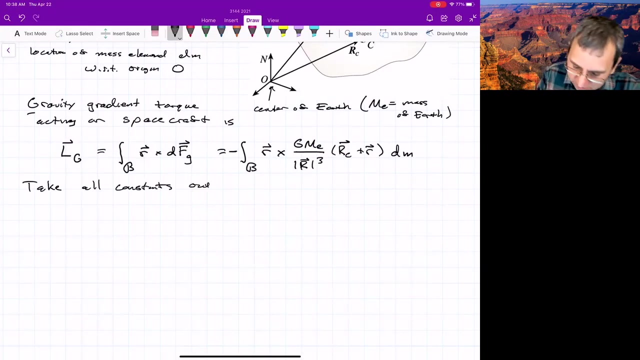 raised to the third. we'll write big r up here as r c plus r, and we're integrating over mass elements. i combined these two to make capital r to the third and then wrote big r for the vector part as r c plus little r. and now we turn a crank of math. if we take all the constants outside the 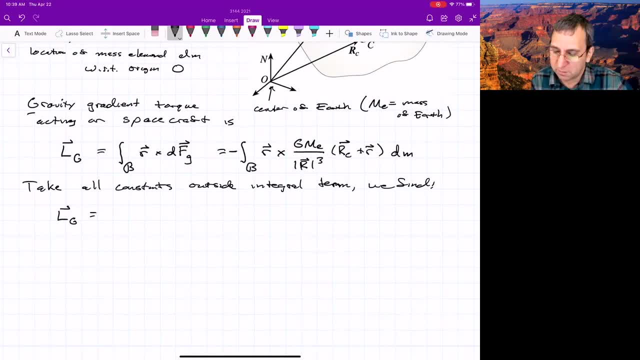 integral term, so things that we're not integrating over. i'm going to flip the order of the cross product of r to the third and then we're going to write big r to the third and then we're going to product. so let me first get g, m, e- that could definitely be brought out. i'll have r, c cross. 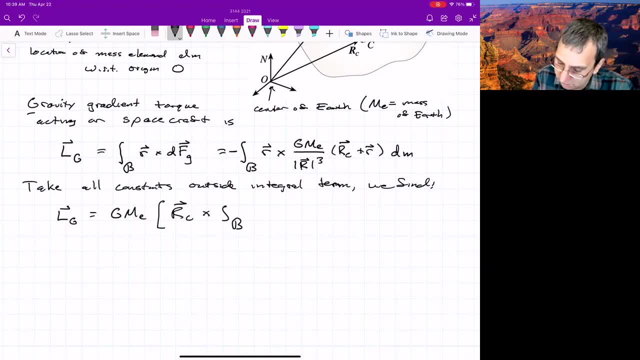 the integral over the body of little r, over big r, cubed dm. and then the other term is going to be an r cross r term. it's going to have r cross r, which is going to be zero, r cross r and over r cubed. we always like fancy ways of writing zero. 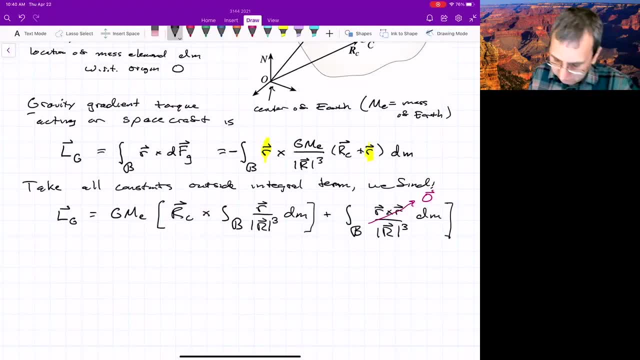 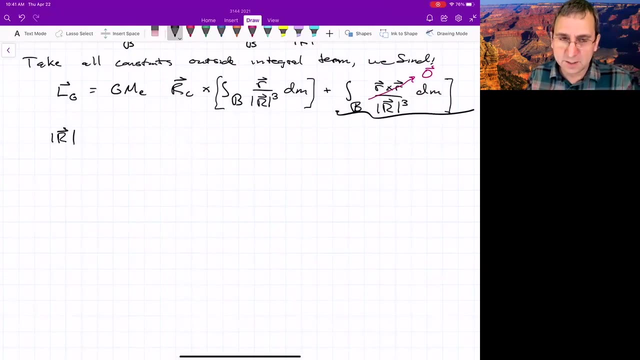 zero, then it drops out. so then we're just left with this term and in fact we could bring out r c, so we're just left with this. so this part just sort of went away and now we need to rewrite the big r to the third. how are we going to do that big r? it contains both r c and little r. a member. 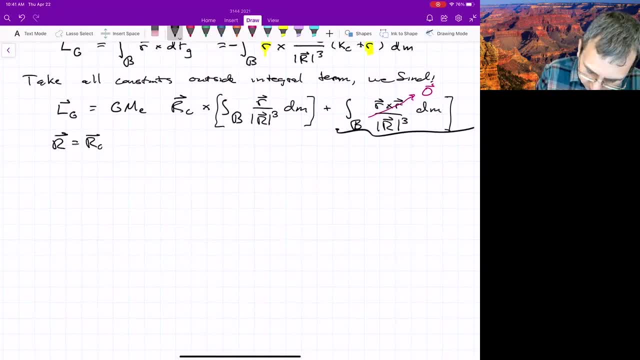 r equals r c plus little r. magnitude of r cubed is actually r c plus little r cubed r squared raised to the three halves. magnitude of r squared could also be written as r dotted with r raised to the three halves, and so this is r c plus little r, dotted with r c plus little r. 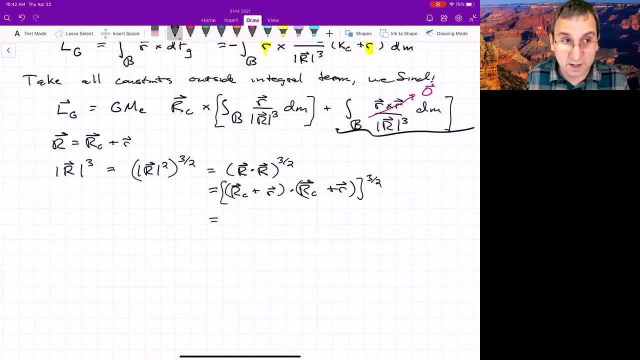 that whole thing to the three halves. you work out what that dot product is, right, you get r c dotted with r c plus, and you'll pick up two r c dotted with little r plus little r dotted with little r, raised to the three halves. well, this is just magnitude of r, this is just magnitude r c squared. but we still have that. 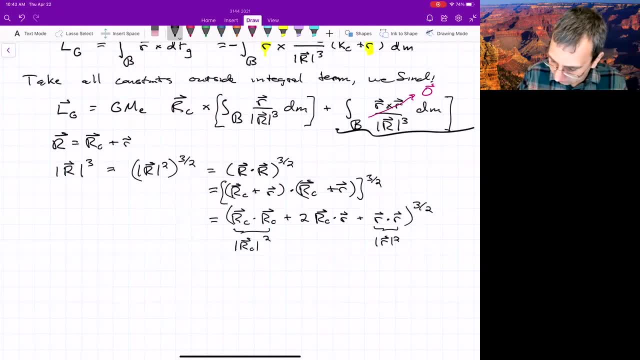 dot product in between. i'm just going to say that magnitude of r c is r c without the vector stuff, and magnitude of r is r. just to make my wife a little bit easier here, so i could write this as the end of the day: r c squared plus two r c, the vector dotted with little r, plus little r squared. 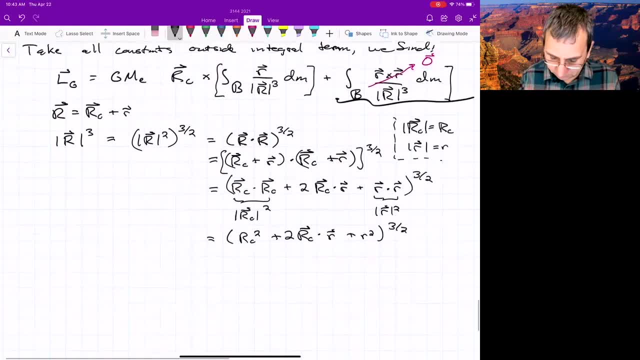 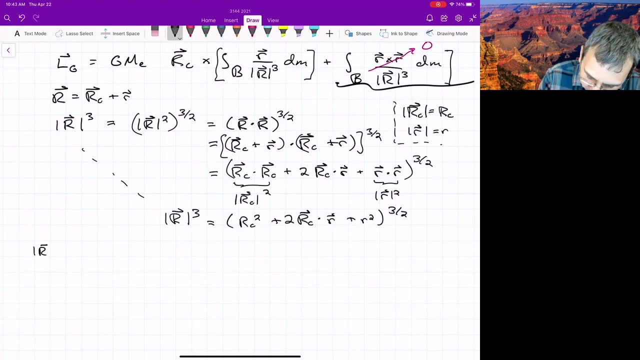 and that's all raised to three halves. what we want is one over r cubed. so remember what this was. if we do one over r cubed, this is just right. one over r cubed. how will we write it? we could write it as: r c squared plus two, r c dotted with r plus little r squared, raised to the negative three halves. 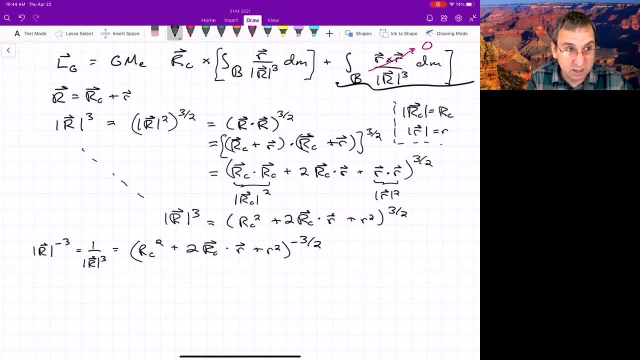 power. pull out the constant which is r c. well, i don't know. constant depends on if this is a circular orbit. let's just bring this thing out. so if we do r c, it's squared and then raised to the negative three halves power. so this is actually going to give us a one over r c cubed we want to do. 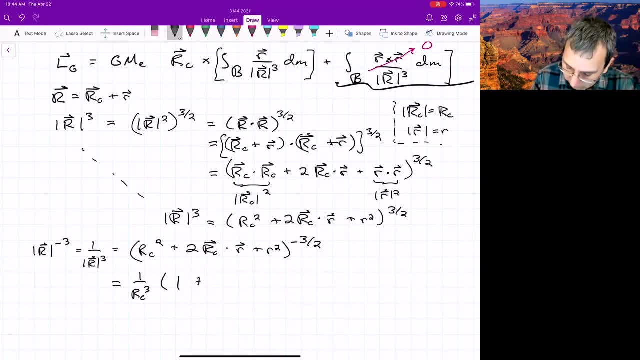 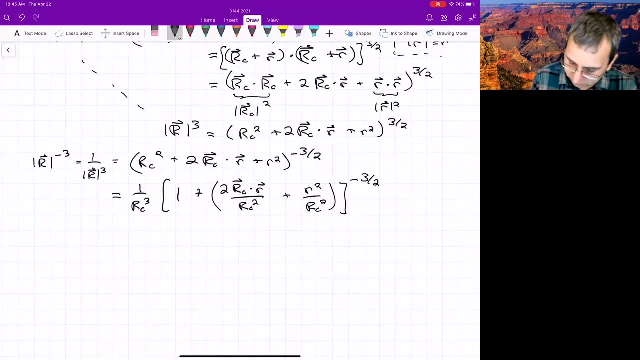 that. so then we have inside this parentheses. it'll be one plus two r c dotted with r, divided by r c squared, plus r squared over little r c squared, raised to the negative three halves power. and now we'll use a taylor series: expansion. i don't know if you've seen this. there's a taylor series. it's good to know. 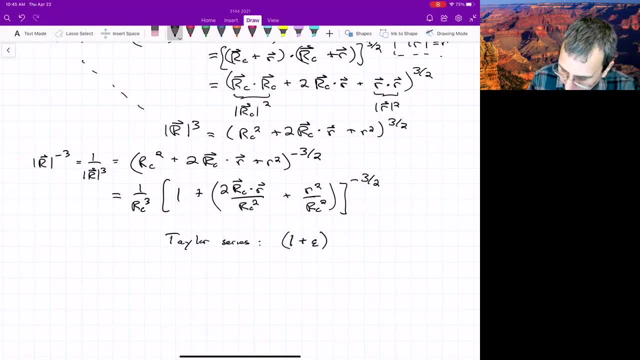 if you have one plus epsilon, where epsilon is small, raised to anything, let's say to the n you need that the magnitude of epsilon is much, much less than one, which it is r. c is big on the order of seven million meters, whereas we're talking about a spacecraft that's on the order of a few. 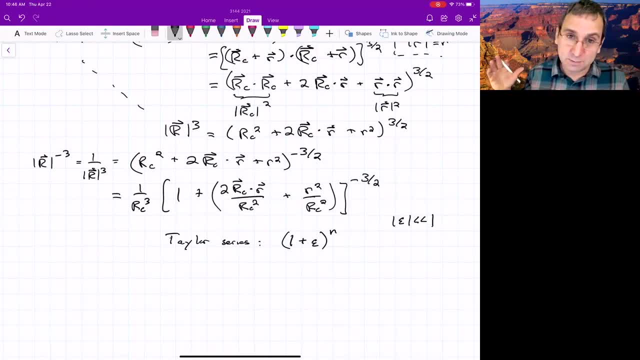 meters. so that dot product is going to be really, really small compared to r c squared, and this one is even going to be even smaller. so we we might even just neglect that. we'll just say this is pretty much negligible. we just want leading order effects anyway. what's this taylor series expansion.